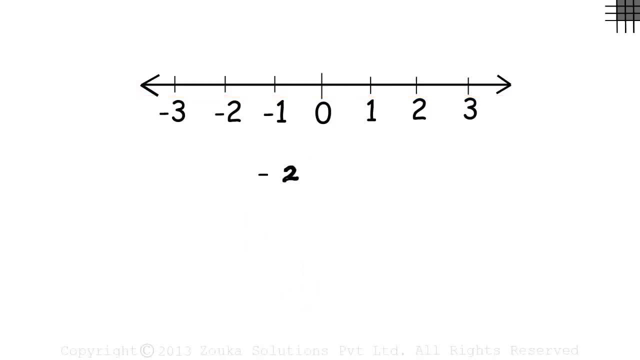 Let's look at a few examples. Say minus 2.. Yes, it can be plotted on the number line. It's this point. So minus 2 is a real number. What about 0.5?? Even though it's not an integer, it can be plotted on the number line. 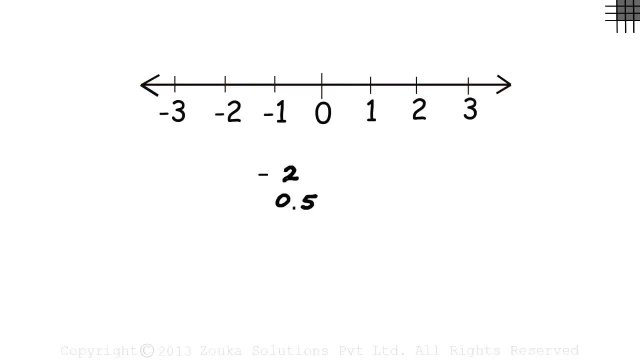 It will be somewhere here. Now let's look at another number, Root 2,, which is also called as square root of 2.. If we calculate the value of root 2, we get it as 1.414 approximately. The digits after the decimal point do not end. 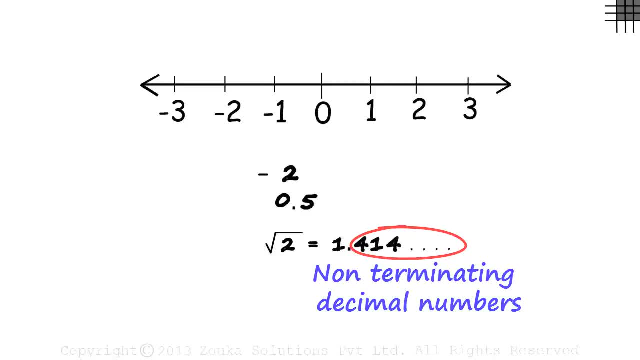 These kind of numbers are called non-terminating decimal numbers, And yes, these numbers too can be plotted on the number line. Plotting a non-terminating number might sound weird, but yes, it's possible. So root 2 is also a real number. 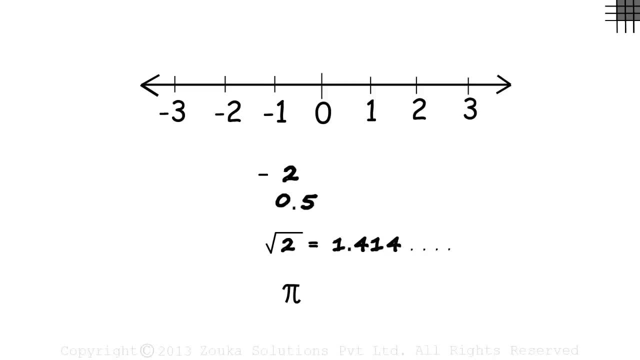 And what about this special number, pi? It approximately equals 3.14159.. Pi is also a non-terminating decimal number And, yes, it can be plotted on the number line, which makes it a real number. So that's our definition. 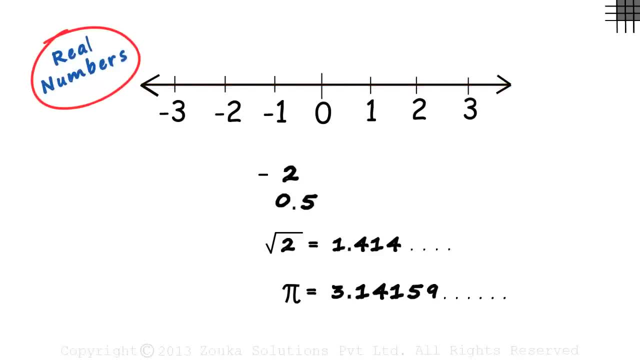 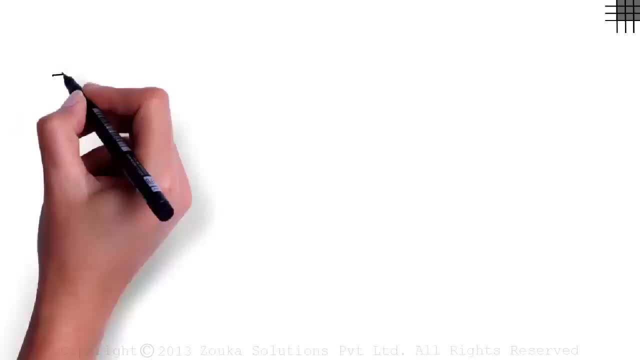 Any number that can be plotted on a number line is called a real number. Now let's talk a bit about the different kinds of numbers we know. The first kind is numbers with terminating decimals, Numbers like 0.375.. The number stops at a point and does not go on and on. 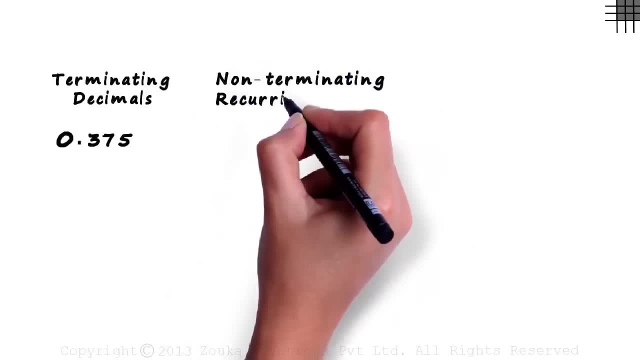 Then we have non-terminating recurring decimals, Numbers like 0.6666 and so on. The sixes don't end. It's called recurring, since the same number reoccurs, And non-terminating, since it reoccurs infinitely. 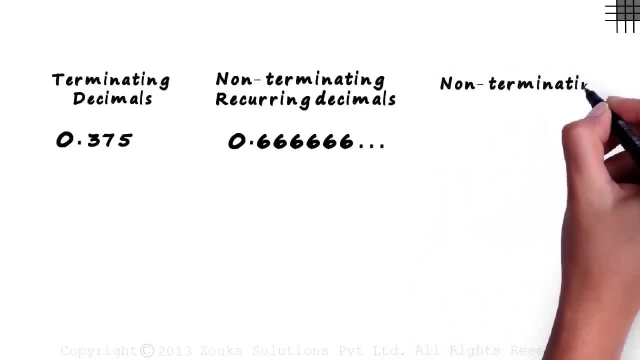 And the third type is non-terminating, non-recurring decimals. We just saw an example of this type, Root 2.. It approximately equals 1.4142 and the digits after the decimal do not end, Hence it's called non-terminating. 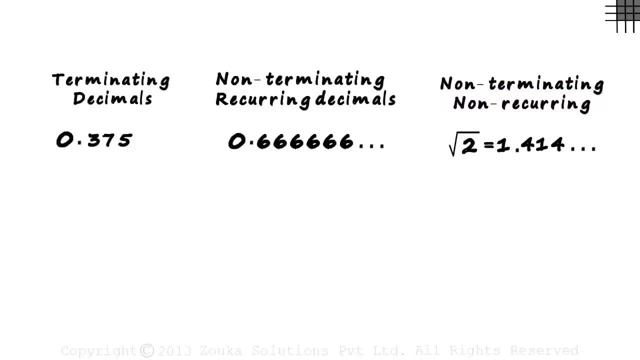 It's called non-recurring, since there is no specific pattern of re-occurrence. Broadly, these are the three types of numbers we see in mathematics: Terminating, non-terminating, recurring and non-terminating, non-recurring.